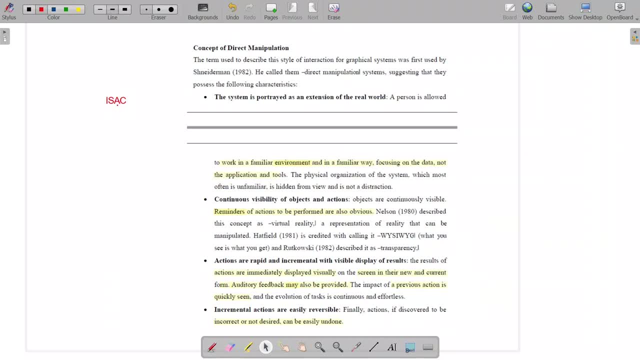 Yeah here. the third question is like concept of direct manipulation and follow characteristics. So what is a direct manipulation? Let's see. So direct manipulation has some characteristics, right. So let's see, suppose, consider some website- okay, some website or ticket as a Aadhaar card, registration or something, Okay. So what happens is so the main thing is like for your purpose, you think you assume that you are going to apply for. 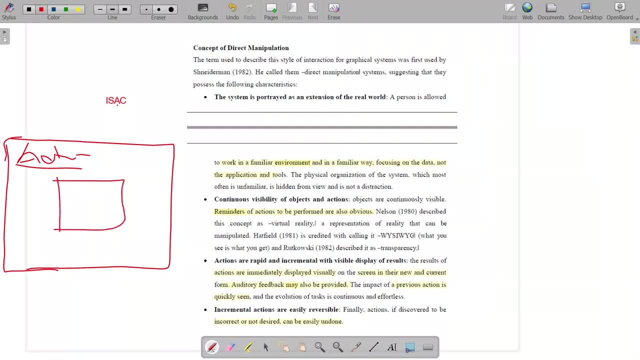 a new form. okay, you're going to apply for a new form, But the main concept is to: you are going to apply, you don't know how you apply or something like that. You're not worried about the applications and the tools over there, You're just worried about the task has to be done. Okay, so your task is to get a new form, But there might be a different options like update address, update number or something like that, And there will be some visibility, right? 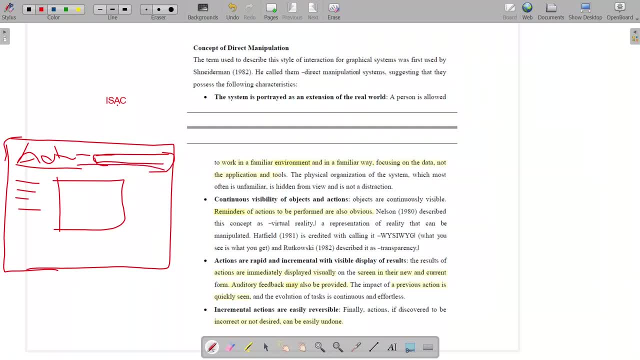 Maybe like update- there'll be some moving object over here- like update your Aadhaar, link your PAN card with your Aadhaar or something like that, And if you've done any mistakes or while filling, you can easily undone or you can go back and update it right. So these are the options. We can say it as a direct manipulation. So these are the following characteristics. So the main key point. I will go from line by line. 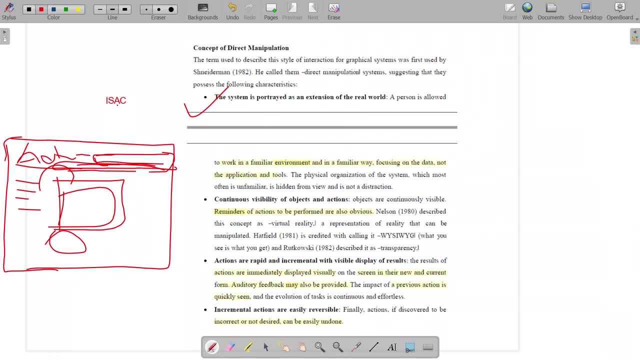 Point by point. So first point: what is the system is portrayed as an extension of the real world. A person is allowed to work in a familiar environment and a familiar way, focusing on the data, not the application and tools. So here you can see that the main, as I said, you are working, you are. the main task is to get your Aadhaar in new form right For Aadhaar. you're applying for Aadhaar as a new candidate, So the main task is, like you work in a familiar environment, in a familiar way, focusing on the data, not on the application tools. The system is portrayed as an extension of the real world. The next: 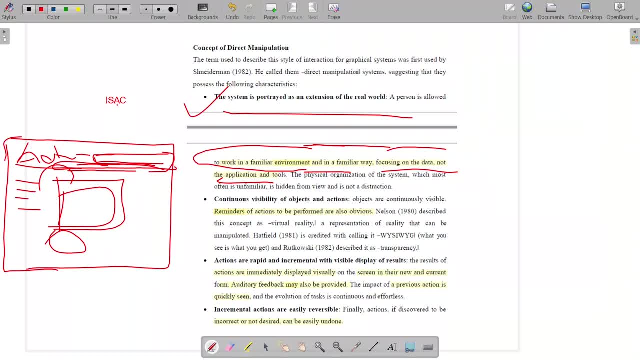 point is continuous visibility of objects and actions. So suppose there are continuous visibility of actions, As I said, PAN, link your PAN with Aadhaar or Aadhaar with PAN or something. Yeah, link your Aadhaar card with PAN. So continuous visibility of objects and actions. Some action you have to take, Reminder of actions to be performed are also obvious, right? The next actions are rapid and incremental with visible display of results. Suppose, if you fill the form one, then there will be other details you want. Like I acknowledge the. 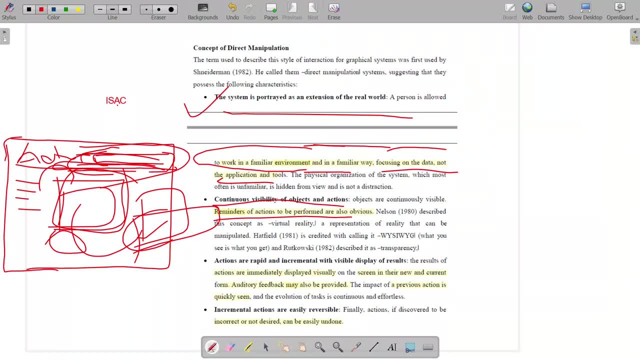 form or something like that in the second page. So this is second page. Like. actions are rapid and incremental with a visible display of result. So whenever you take some particular action, the immediate action it should be take, Like if I give a submit button, it should not take a lot of time to get submitted. It should submit within seconds, Okay, which is a few seconds. Okay, it should be like that, So your actions are immediately displayed visually on the screen. They're new and current form. Auditory feedback. 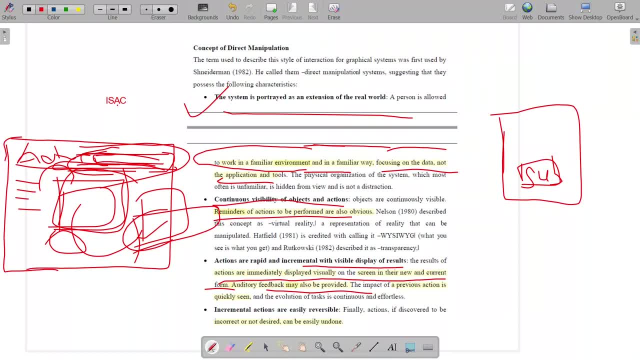 may also be required. Suppose, once you fill the form, then you have to give some feedback over there, Like, yeah, I have done this in a better way or than the previous thing, like that. So then the last one is: incremental actions are easily reversible. Suppose you entered a data wrong. Okay, suppose you entered your mobile number wrong, Like you added 11 digits or 12 digits. You have to go back and update it soon. Like you can have the. 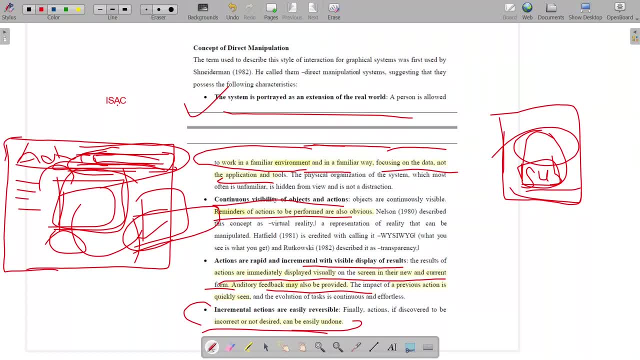 option that you can update. That's what the good design works like. That's how good design works. So what is the keyword over here? The keyword is ISAC. So I know the ISAC spelling is I double S A C, But for keyword I S A C. This is a keyword for the direct manipulation. So what is I? I is incremental. Incremental actions are easily reversible. Just write the main point and this the highlighted one: Incremental actions are easily reversible.